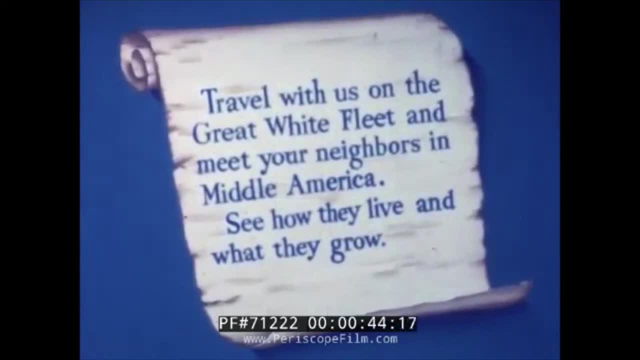 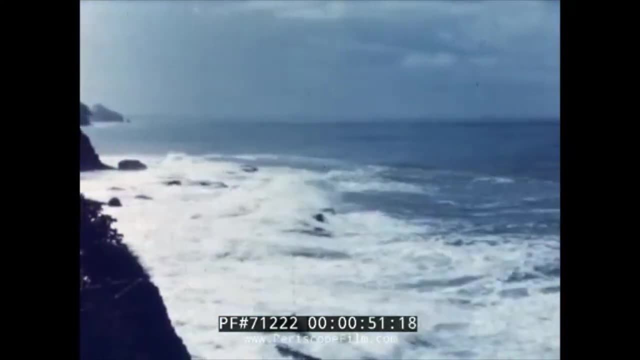 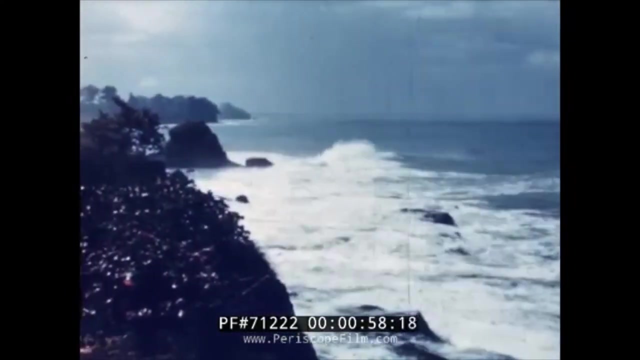 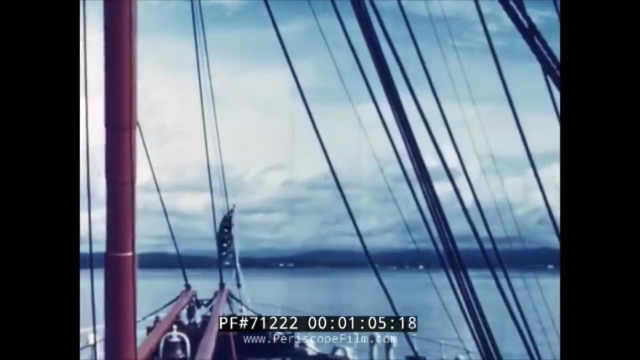 it to the United States and Europe. A thousand miles south of New Orleans, the blue waters of the Caribbean break upon the shores of Central America. For many years, these fascinating tropical countries have been served by United Fruit Company's great white fleet. These lands are principally agricultural. 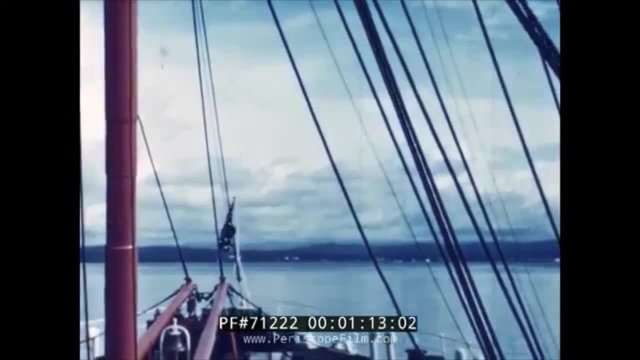 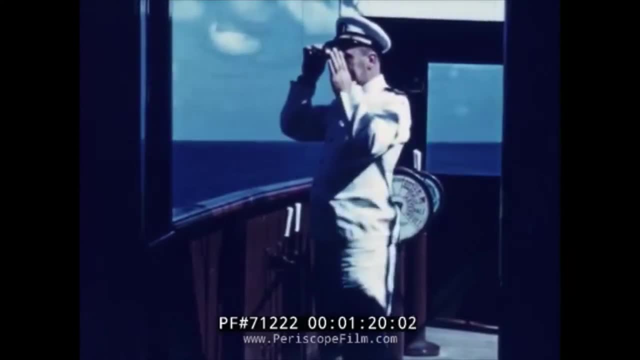 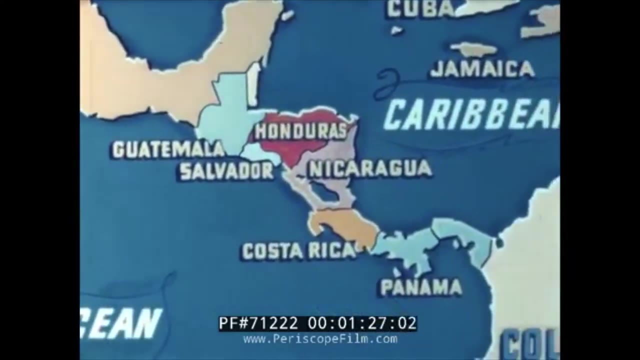 and their combined population is actually less than the population of New York City Bounded on the north and Columbia on the south. Central America includes Guatemala, Honduras, Nicaragua, El Salvador, Costa Rica and Panama. Add to this area the important island republics. 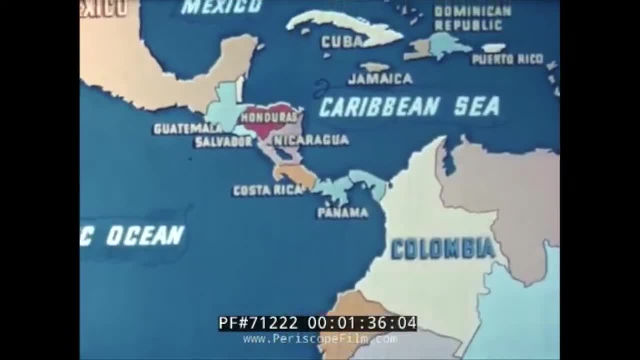 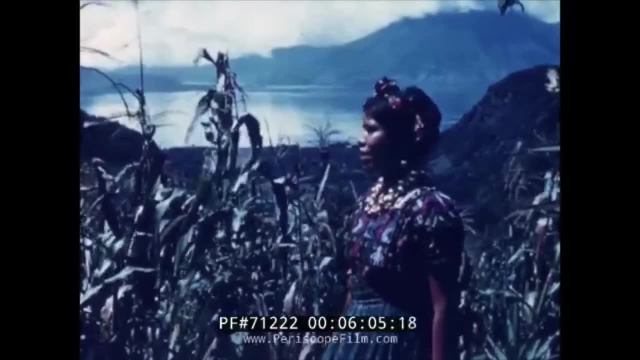 of Cuba, Haiti, the Dominican Republic and the British island of Jamaica, and you have encompassed the area known as the United States. The United Fruit Company had enormous impacts on the political and economic development of Central America, while enhancing corporate profits at the expense of small farmers' security. 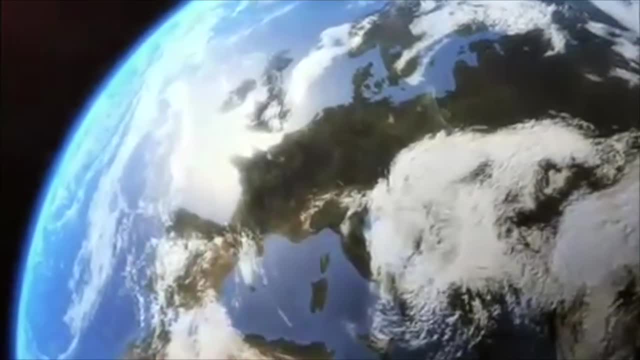 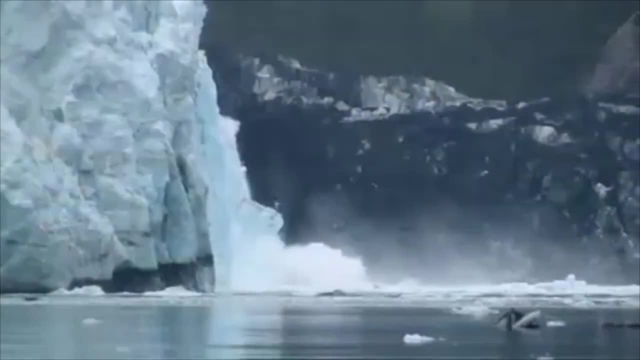 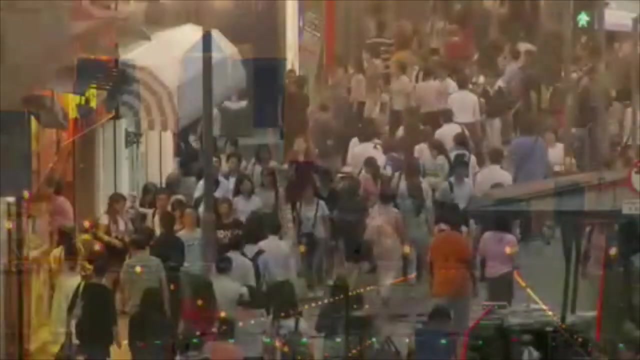 Global environmental justice has developed as a rhetoric within the past few decades to combat the unjust impositions of environmental burdens on marginalized communities and nations. Due to an increasing globalized and neoliberal economy, countries in the Global North have experienced increased profits at the expense of the Global South. This can be seen through: 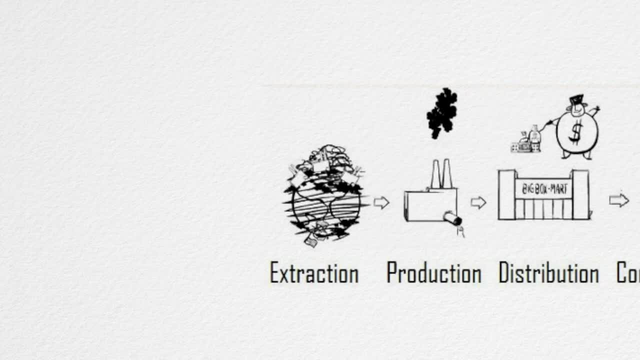 processes such as the treadmill of production and consumption, in which affluent consumers in the North partake in a capitalist consumer society and in which affluent consumers in the United States are exposed to the effects of the global economy. The United Fruit Company has become the most important consumer of the country, and the United Fruit Company has 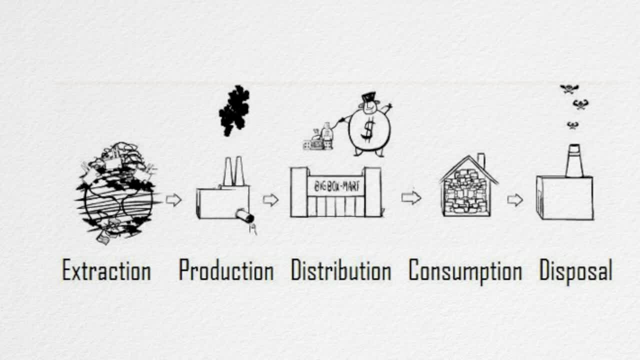 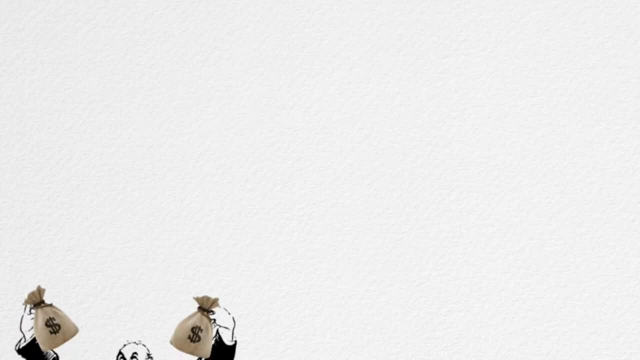 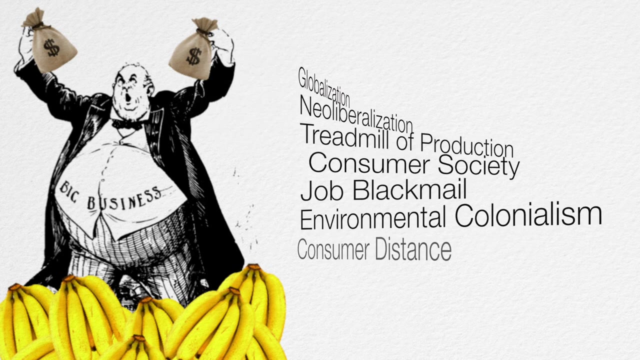 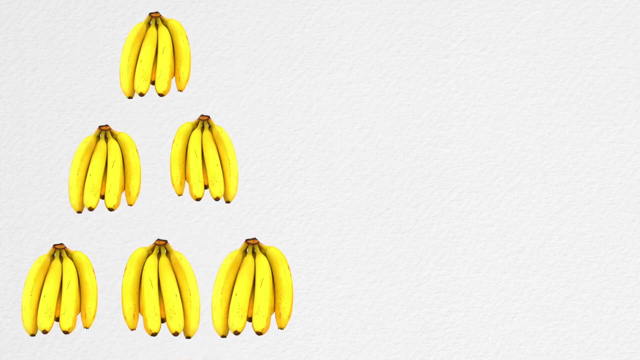 demands new disposable goods, while developing countries and marginalized communities shoulder the waste and pollution that is produced Within the global banana production complex. there are several theories, structures and processes of global environmental justice. The first example is that of job blackmail, in which consumer demands cause decreased wages as a product. 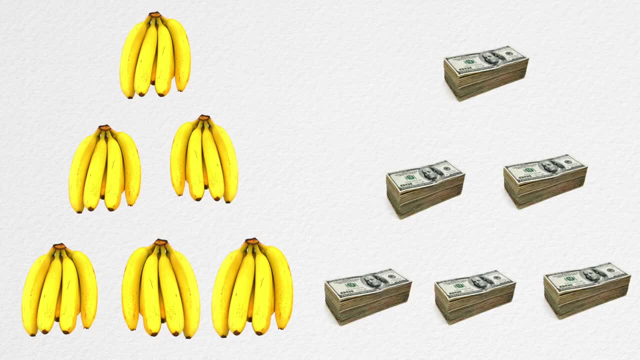 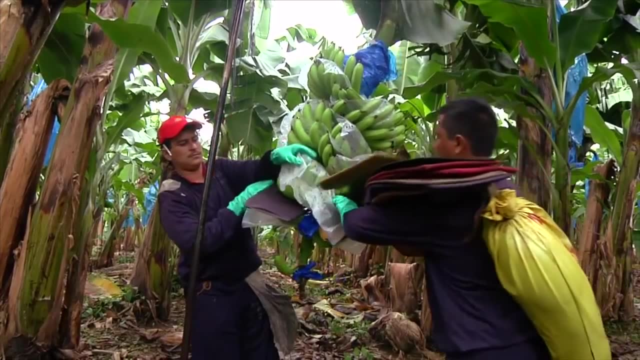 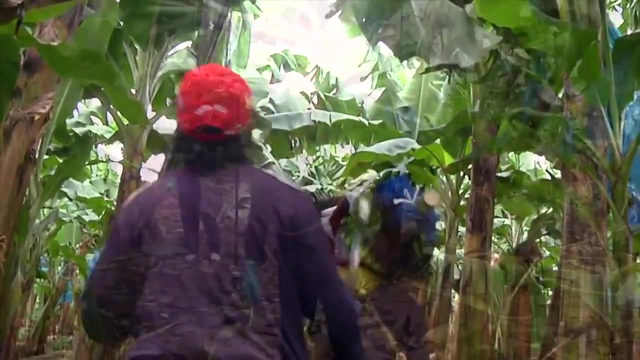 becomes cheaper. Because of this, workers must engage in increased risk for lower wages and more hours of work. Workers face constraints that force them to accept their risks of pesticide exposure. These constraints include limited job options, a weakened union presence and systematic failures at the judicial 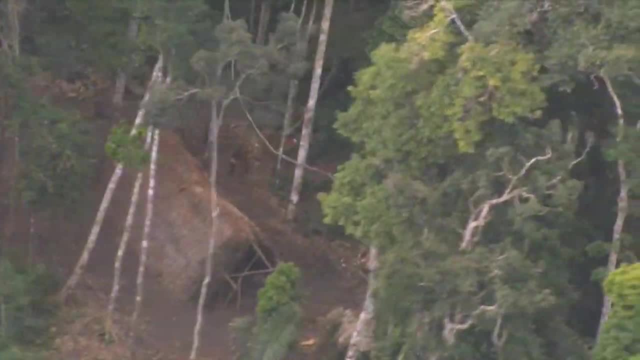 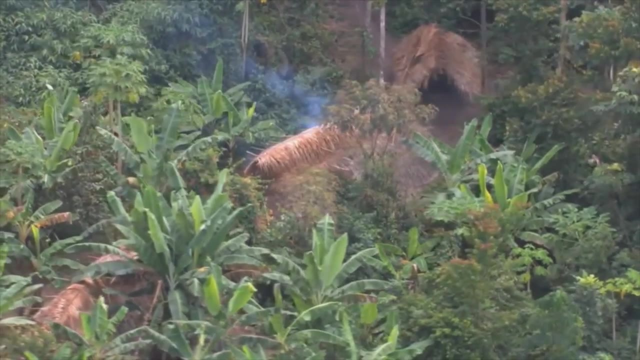 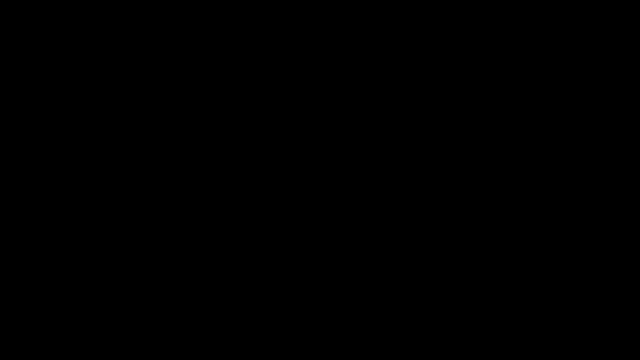 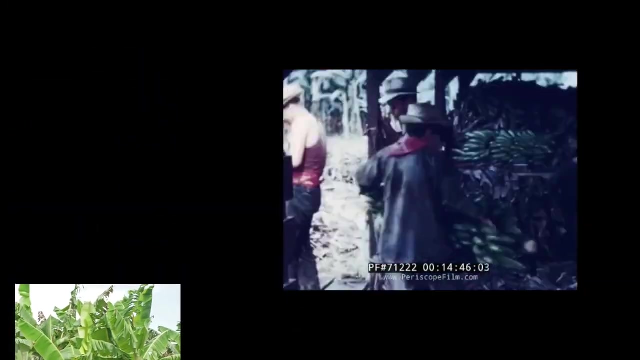 level. Environmental colonialism can be seen through the repeated foreign subjugation of indigenous peoples and environmentalists In an effort to extract natural resources. This reproduces the colonial era dynamic of foreign profit as a result of oppressing native people. It is interesting that while we think of the banana as a hearty food, this is only 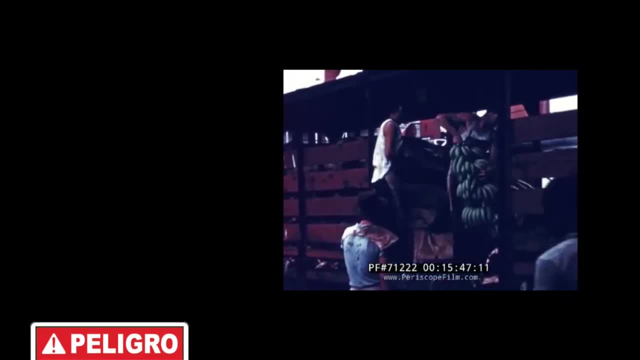 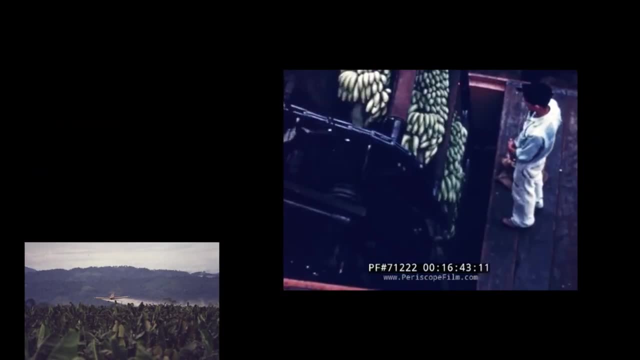 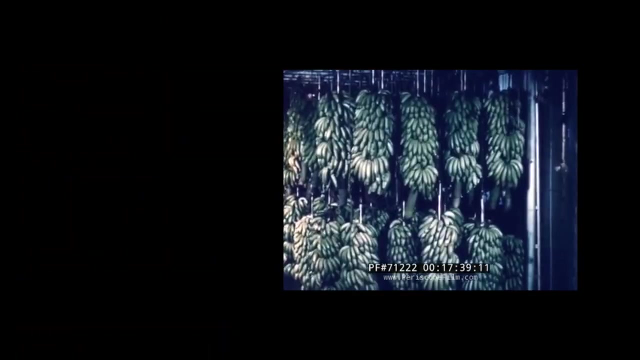 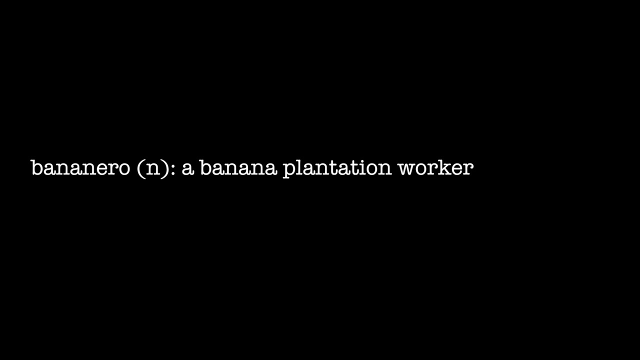 because so much care is taken to see that it arrives on our tables in good condition, For the banana must be cut green and ripened artificially. It is one of the few fruits that loses its flavor if allowed to ripen on the plant. Bona Narrows banana plantation workers face a number of health threats by working in. 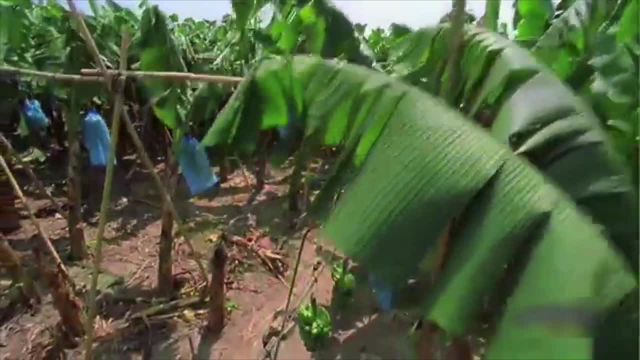 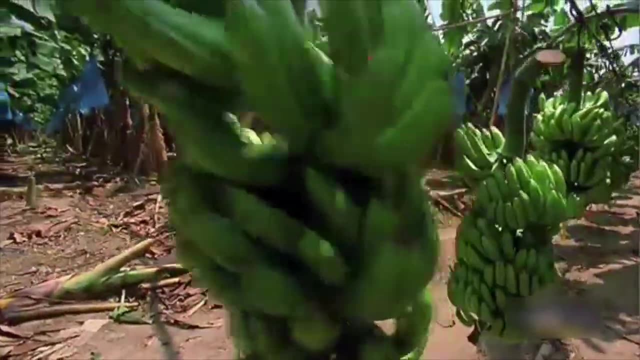 monocultural banana fields. Chemicals are applied to the banana plant at every stage of growth: First herbicides, nematocides and then fungicides. In a These chemicals are often encased in the plastic bags. workers must put on stocks and then remove. 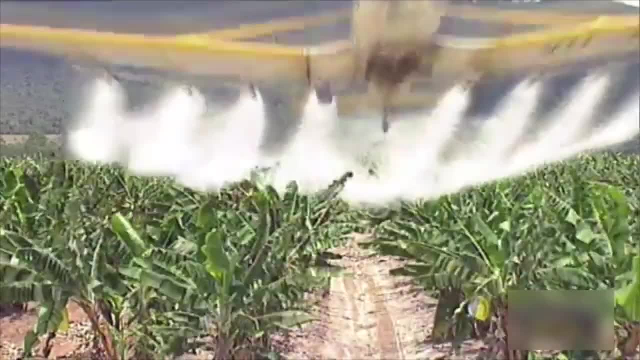 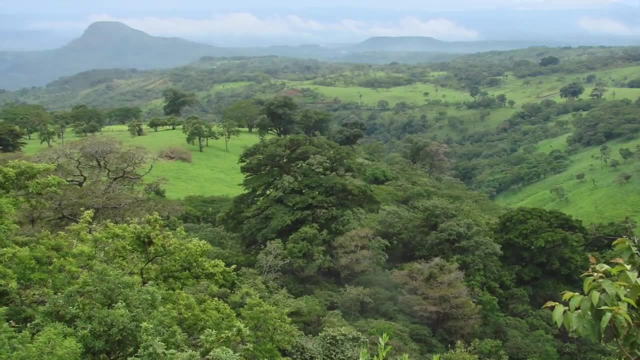 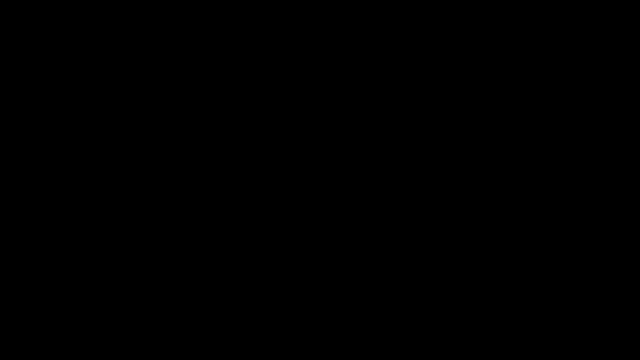 and dispose of Pesticides and fungicides, are also often sprayed aerially. All of these chemicals can be washed off of plantations because of high rainfall averages and are then taken into groundwater systems that can affect entire communities. These bananeros, often untrained and marginalized workers, lack sufficient precautionary instructions. 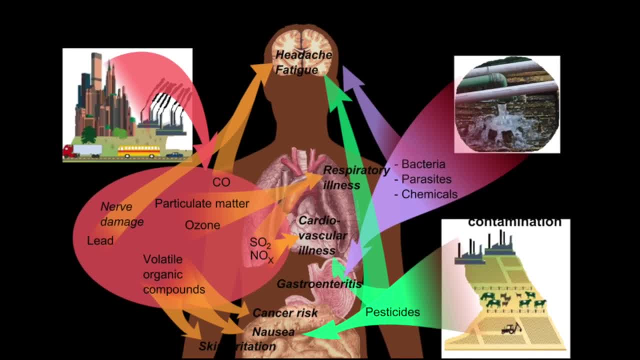 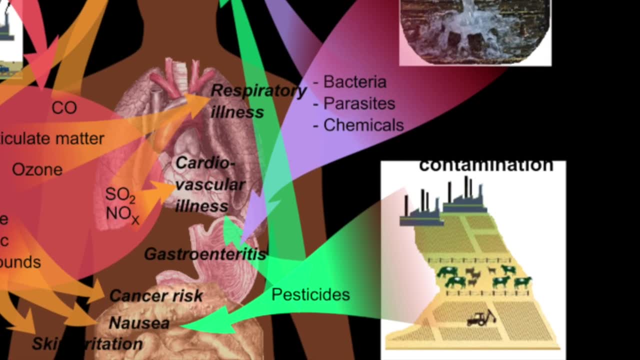 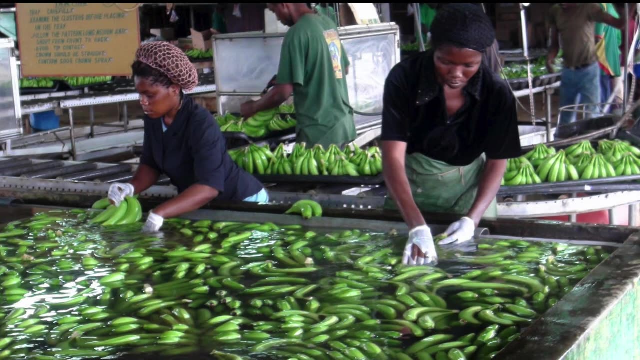 or protective equipment. The chemicals used in banana production are not approved under the US EPA guidelines and can have a negative effect on the respiratory, endocrine and reproductive systems. Women in banana packing plants have complained about skin lesions and headaches while field.